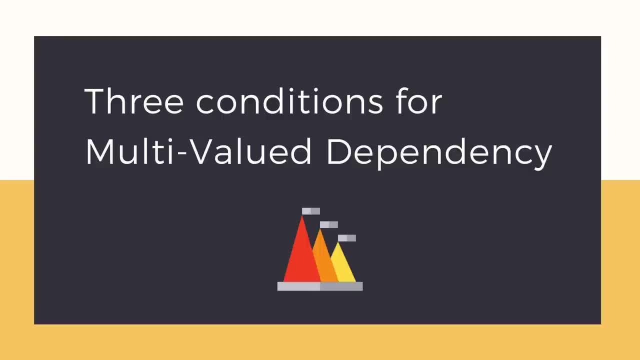 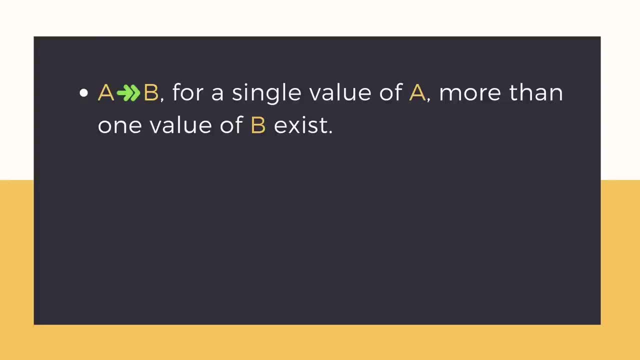 occur together leads to multi-value dependency, and they are for: A derives B. if for single value of A, more than one value of B exists, table has at least three columns, and for a table with columns A, B, C, if A and B have a multi-value dependency, then B and C should be independent of each other. 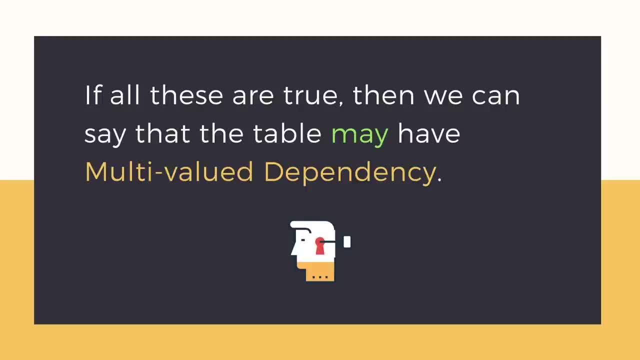 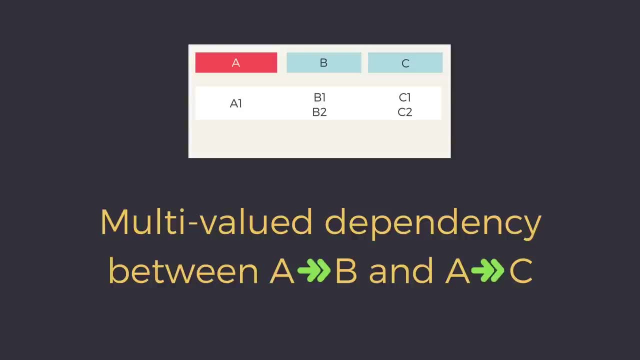 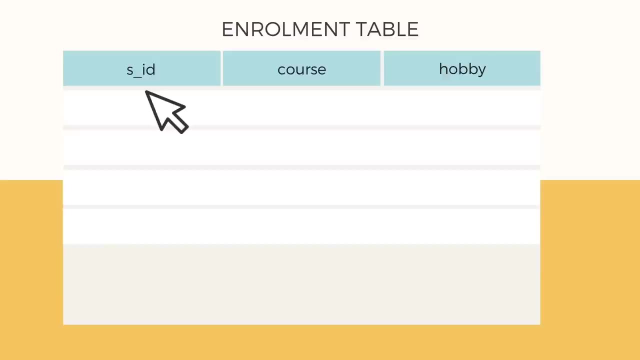 If all these are true for a table, it will be having a multi-value dependency. Also, in a table, multi-value dependency can exist for more than one columns too. Let's take an example to clear all the doubts. So we have a table with S ID. 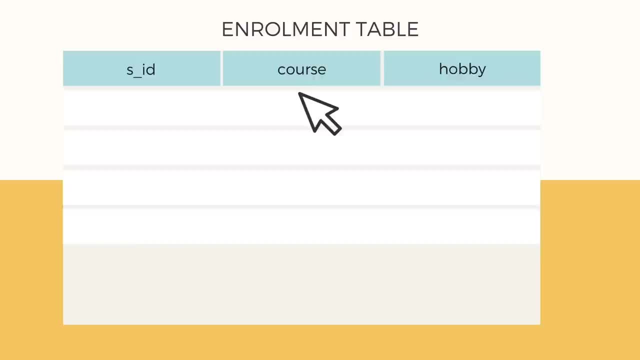 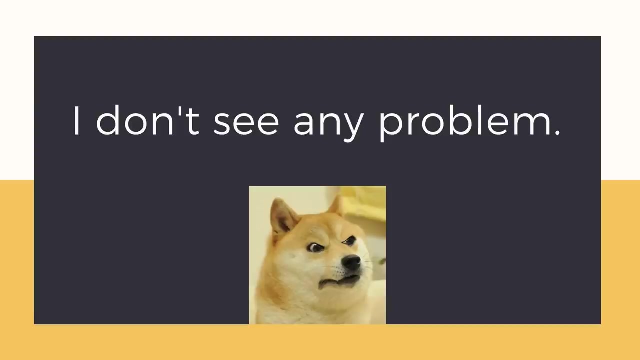 which is student ID course, which is the course opted by the student and the hobby of the student. Let's add data to our table. As you can see, one student has opted for two subjects and has two hobbies. You must be thinking what problem this could lead to. Well, student with S ID 1 has hobby cricket and hockey. 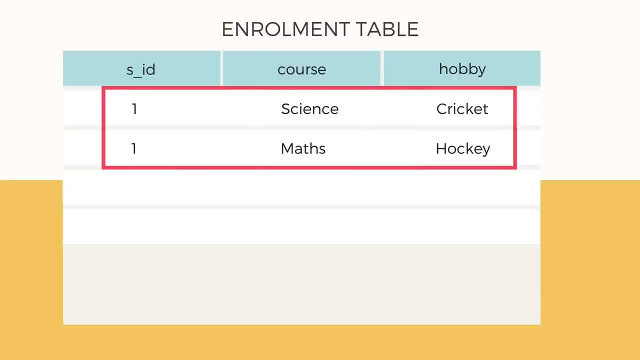 and has opted for subject science and maths, These two rows of data will give rise to two more additional rows. Isn't that right? And there is no relationship between course opted and hobby of the student. Hence it's always advised to keep such attributes in separate, independent tables. Now this can be. 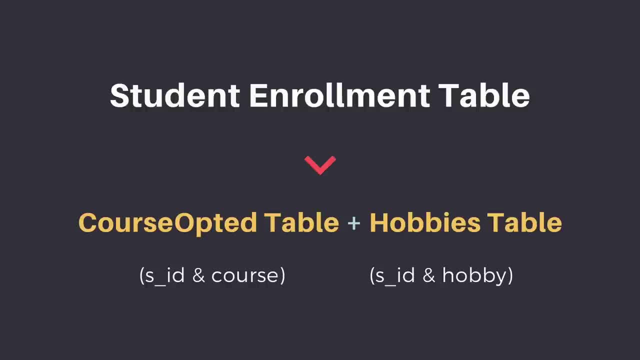 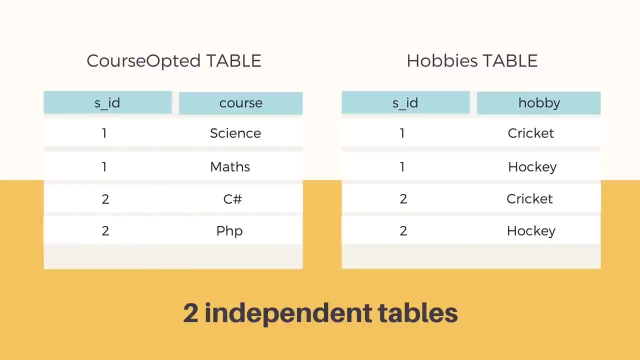 decomposed into two tables to solve the problem of multi-value dependency and to make this relation satisfy the fourth, normal form. This is how the decomposed tables will look like, with student ID and course in one table and student ID and hobby in a separate table. In some cases a table can have functional. 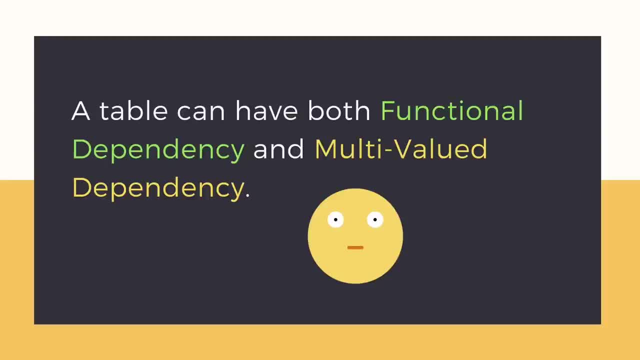 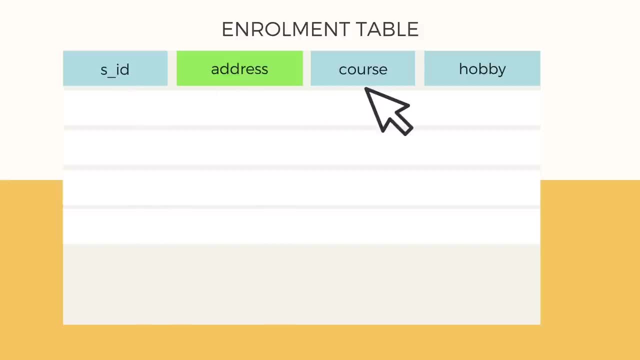 dependency and multi-value dependencies together. For example, if we add address to our table, our table will look like student ID, address, course and hobby. Clearly, address of student will be functionally dependent on S ID, while we have multi-value dependency between S ID and course and S ID and hobby. So this table will be decomposed into three tables to